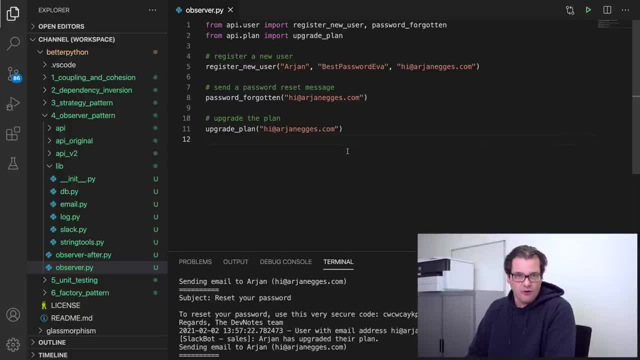 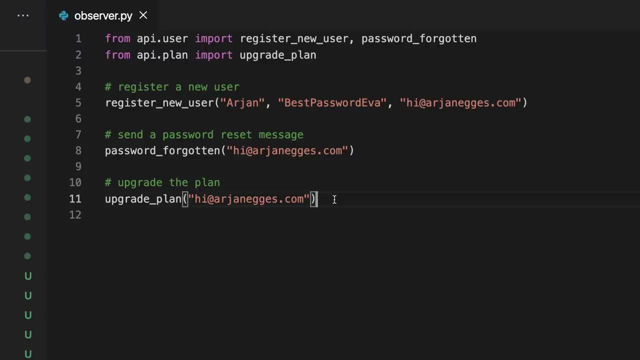 structure of this example. This sample is a little bit more involved than the previous ones because I wanted to show something that kind of approaches the situation like you would encounter in real life. The example that I have here imports a few functions from an API folder and it does a few things. 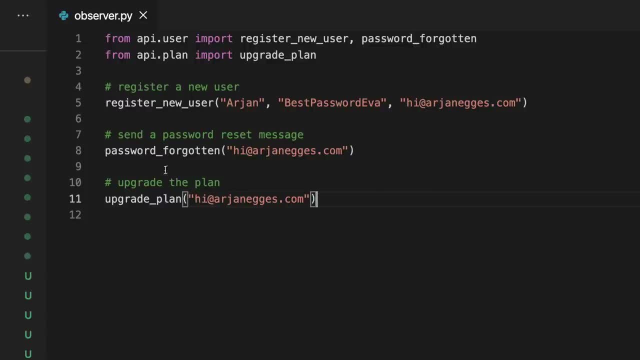 It registers user, it sends a password reset message and upgrades the plan of a user. Now, normally these things would be API calls. I just put them right here in the code, just for testing purposes. If you look at the API folder, we have a. 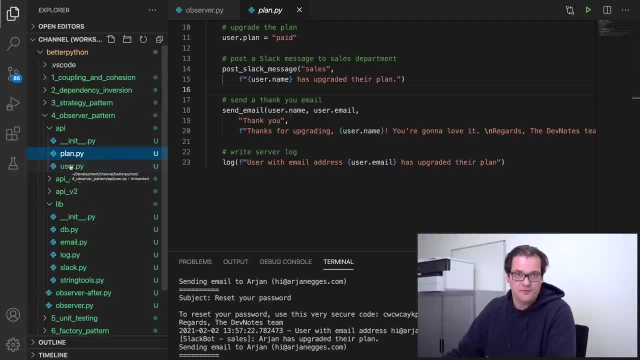 user pinned name. We just drop an API one here just for testing purposes. Now, if you look at the API folder, we have a user file and the plan found these actually contain the methods that I was calling just there. so in user, for example, we have to register new user, which takes a. 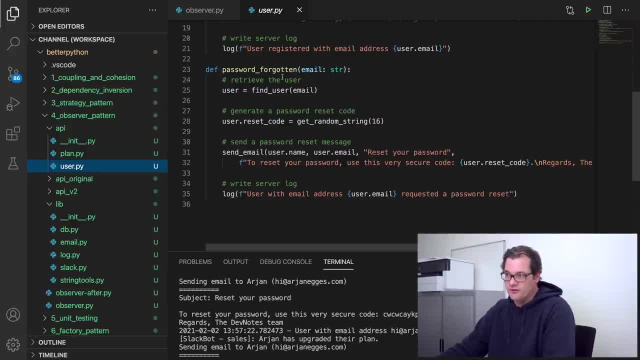 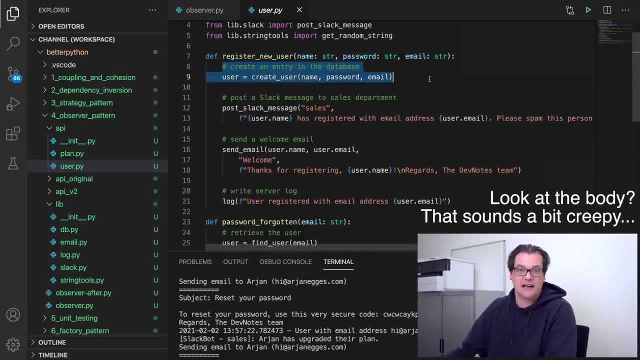 name, password and email address and we have a password forgotten function that takes an email address. so if you look at the body, there's one part which is actually the actual job that it needs to do, like creating a user, and then it posts a few messages, like here: it posts a slack message. so the sales department. 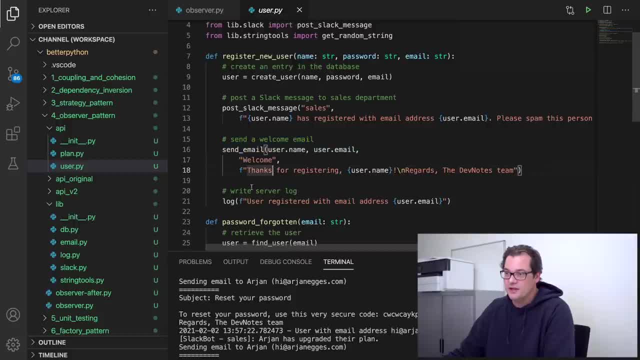 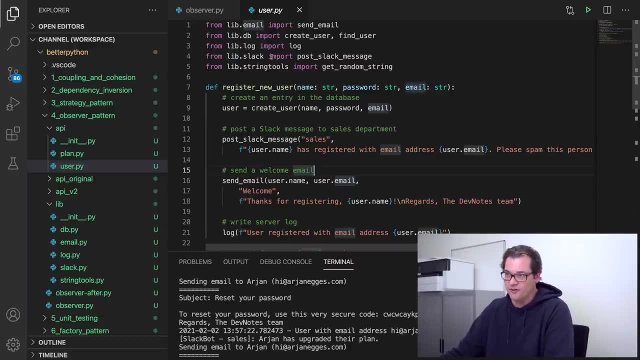 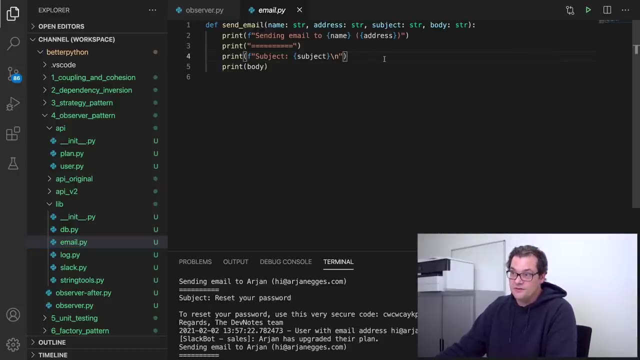 can spam the person. it sends a welcome mail, it writes something to the server log, etc. etc. and these things are all imported from a lib folder. at the moment, this doesn't really do anything like. for example, this sent email message doesn't actually send an email, but it simply prints the message to the console. 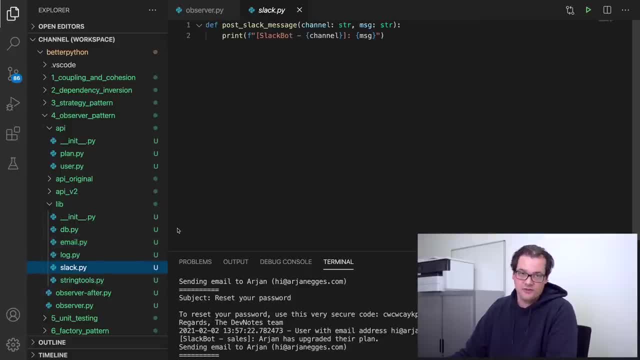 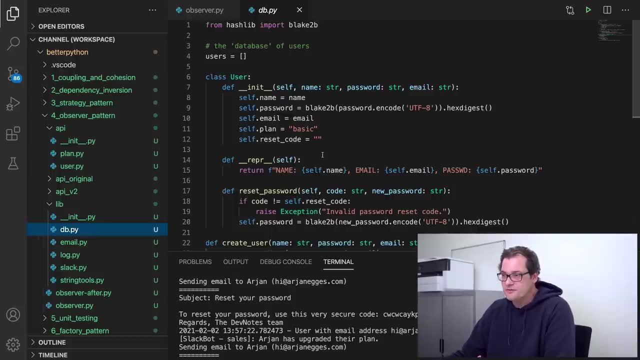 similar for log and for slack in a real application. obviously, these would be integrated with the actual services that you'd be using. the database is the most common application in the world and it's a very complicated application. and it's complicated of all these things in the sense that it's also not a real database. 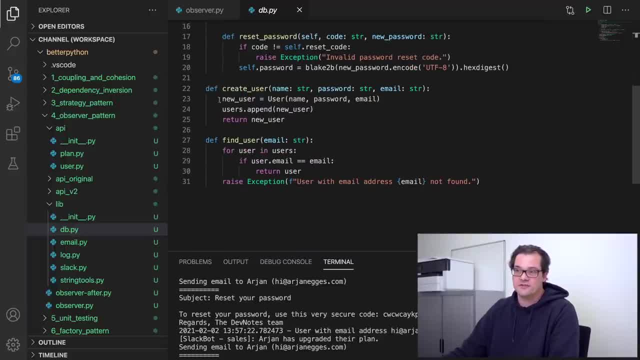 but it creates an array of users. it has a class user that has name, password, email and a few other things, and then it has a few functions, so you can create a user and you can find the user. these are things that you'd normally have in a 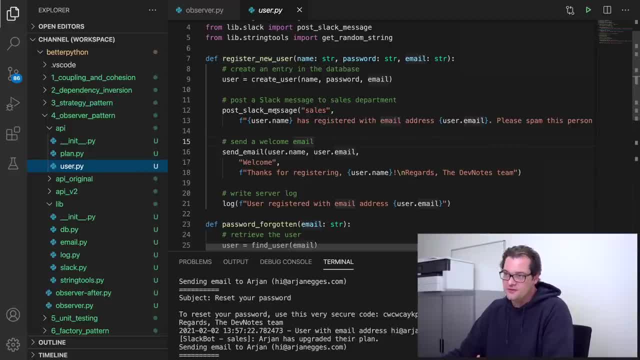 database driver, but here in this example, obviously we're just doing that locally. now the problem with this code is that if you look at, for example, register new, it's overall a method that has pretty weak Cohesion. not only does it need to know about database stuff, it also needs to know about slack, email logs, Etc. now 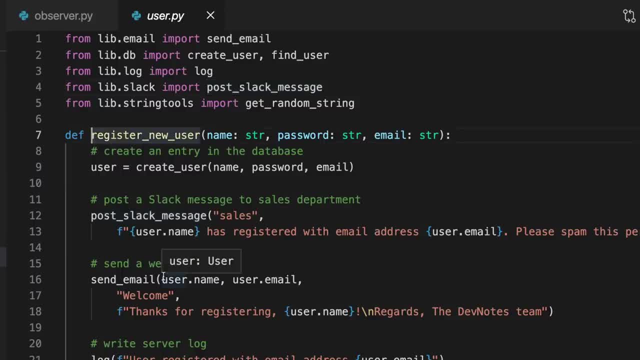 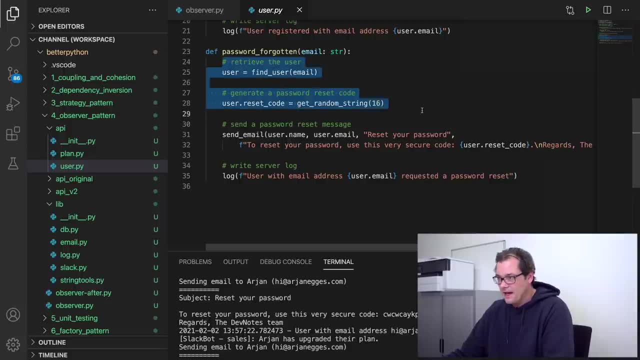 because register new user needs to know about all these particular functions. it means you also have a lot of different imports here and similar for password forgotten. so it also does the actual job it needs to do, which is find the user and generate a password reset code, and then it sends a message. it writes something. 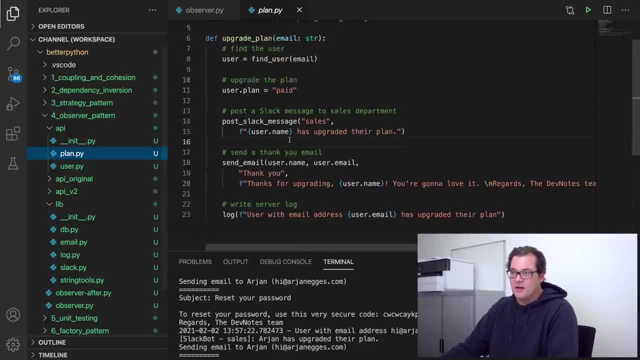 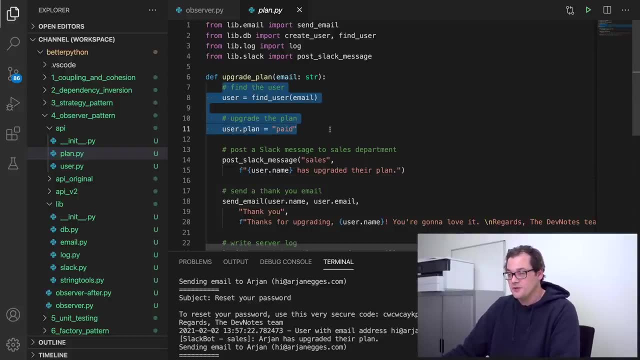 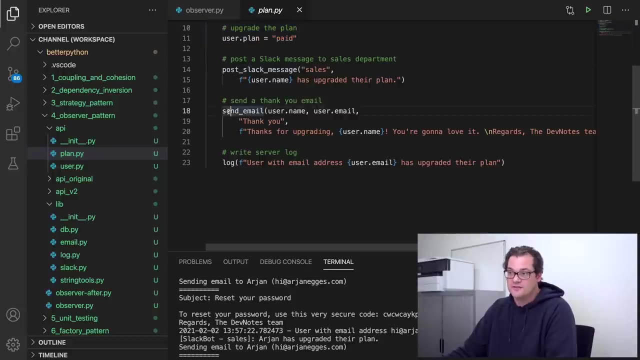 to the server Etc, Etc, and for the part of the application dealing with upgrading the user's plan, it actually looks pretty similar. part of this job is doing the changes in the database, which is, finding the user, and then upgrading the plan in the database, but then it also posts a slack message, sends an. 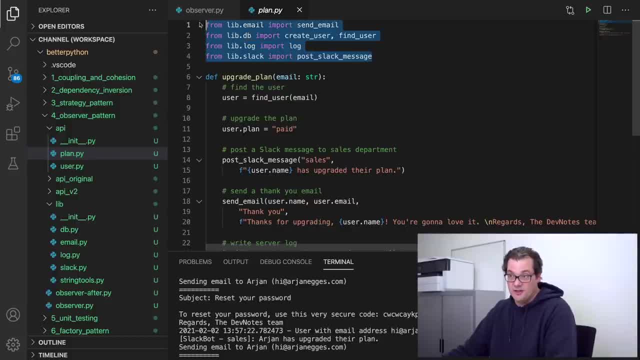 email, write something to the log, and you see also here there's a lot of different imports. that means that upgrade plan, just like register new user, also has pretty weak Cohesion and it's directly coupled with all these very particular implementations. so that sounds very nice and we want to change that. and this is where the observer 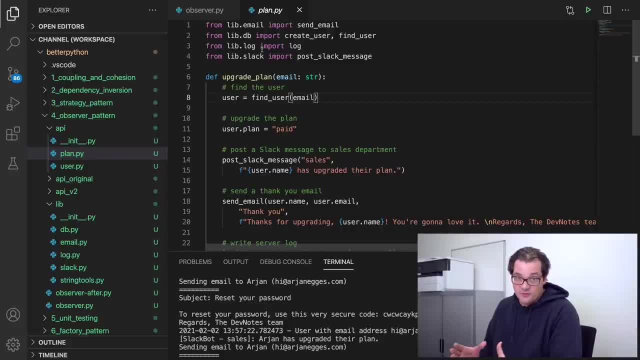 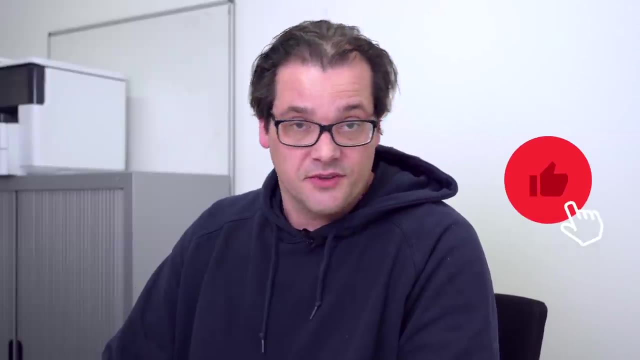 pattern or, specifically, an event system, can really help you separate these things. so let's try to rewrite this application so that it uses events instead of these direct couplings between the code and the messaging. python has several event libraries, but just to show how it works, I'm 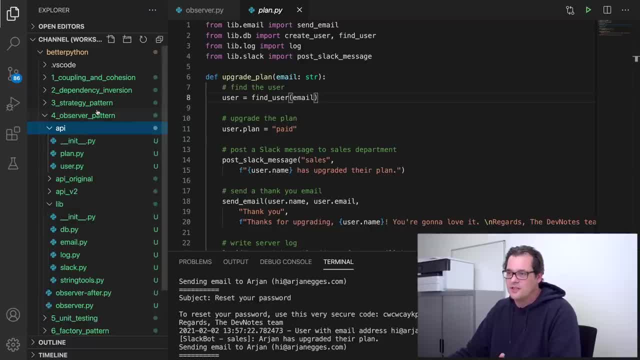 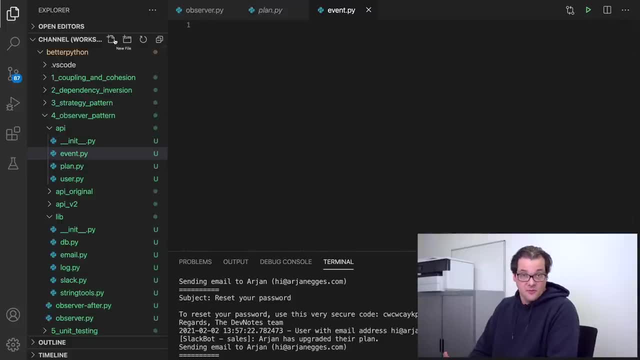 going to write my own. it's. it's actually pretty simple, so let's add an event file here, eventpi, and basically the event system is very simple. you have a number of subscribers that subscribe to different types of events and whenever you post an event, you need. 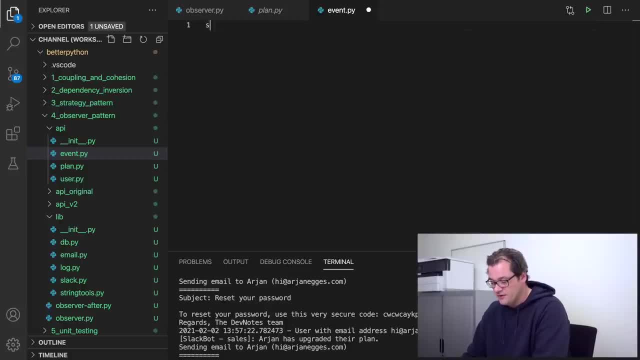 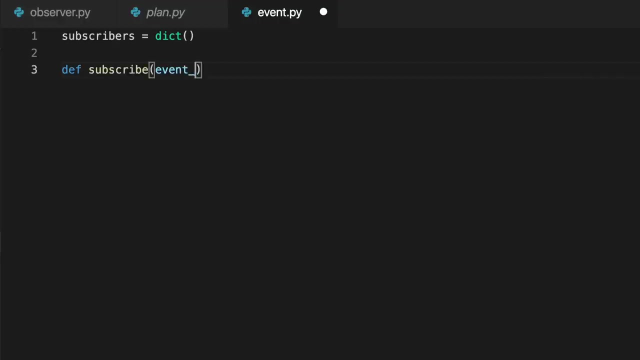 to notify the subscribers. so let's create first a dictionary containing the subscribers and we have a dictionary, and then each item in the dictionary is going to be, for that particular type of event, the list of subscribers that need to be notified when that event happens. so let's add a subscribe method that does that for us. so we're giving it an event. 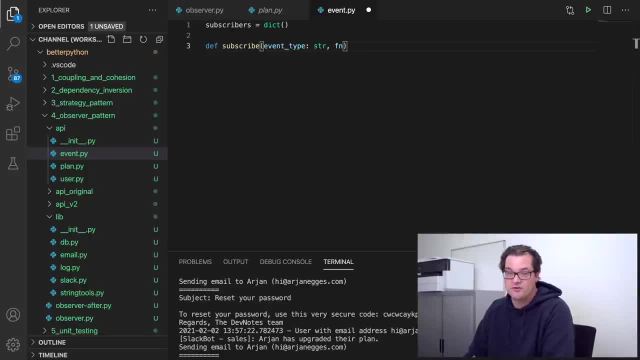 type, which is basically just a string and a function that needs to be called. I'm not going to use type hints here for the function because, frankly, in python type hints for functions are a complete mess, the only thing we have to do when we subscribe to a particular event type. 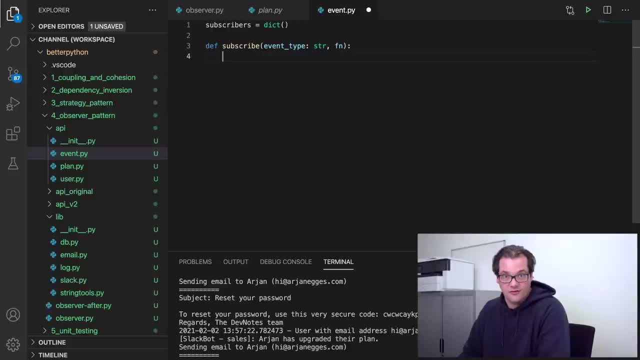 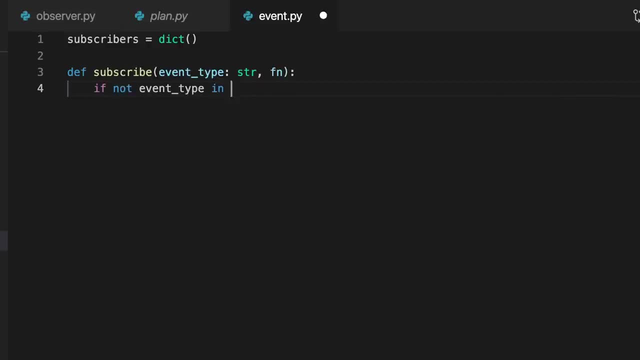 is first check that there is already a list of that event type in the dictionary. so we need to create one and then add it to the list. so if not already in subscriber list, then let's create a list of subscribers for this particular event and we're directly appending the function that needs to be called to the subscriber list. 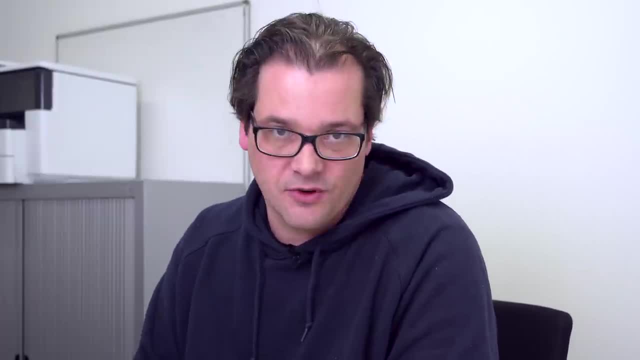 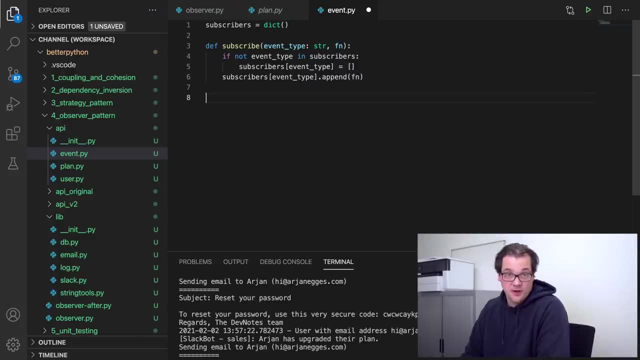 now again, there are already event libraries, so you won't have to write this yourself. I'm just adding it so it shows you how the pattern actually works. and then, next to subscribing, we also need to be able to post events, so let's add a function for that as well. 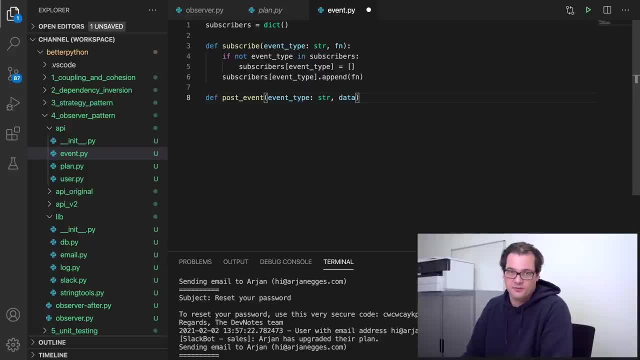 and normally when you post an event you generally want to pass along some data with it. so if there are no subscribers, if the event type doesn't exist in dictionary of subscribers, then we don't have to do anything. otherwise we're going to go over the entire list of subscriber functions and 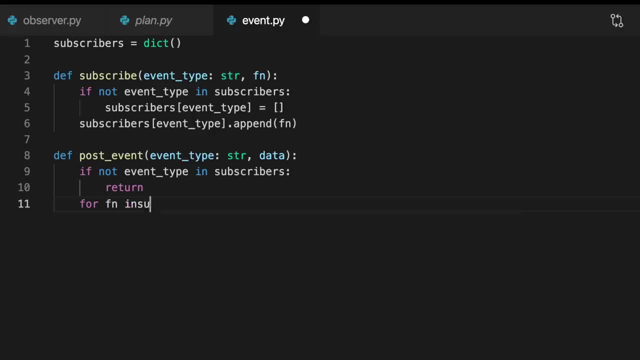 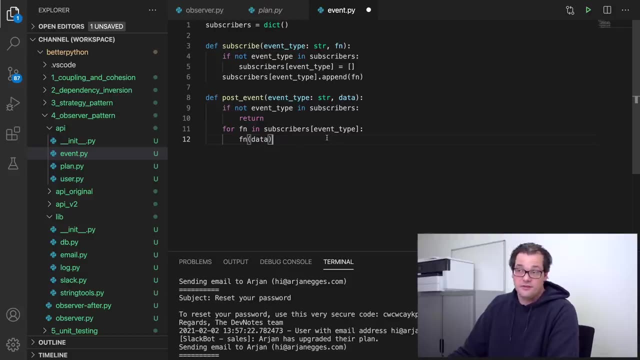 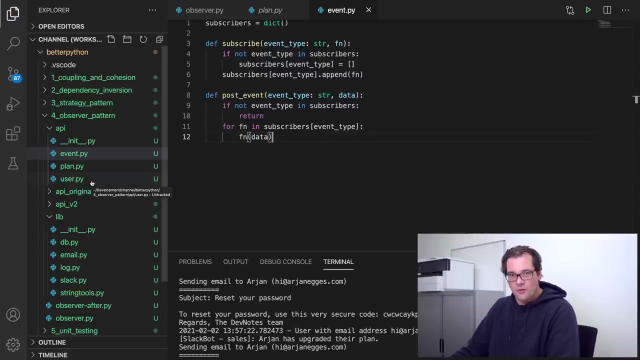 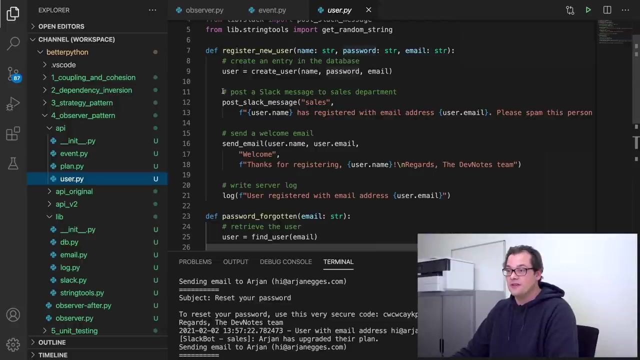 call each of those functions with the data. so there you have it. this is actually a complete- well, almost complete- event system, and this actually works just fine. so now what we can do: we can go back to, for example, the user functions like registering new user, and then replace all this stuff with simply a posting an. 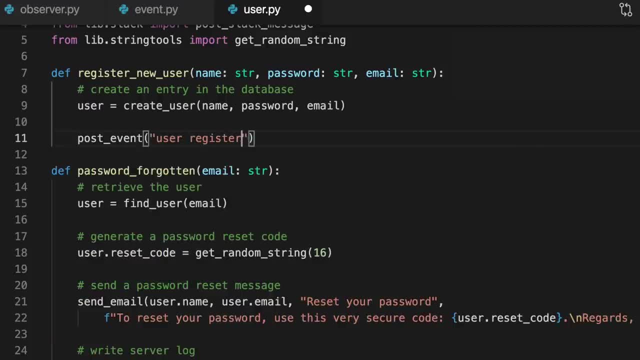 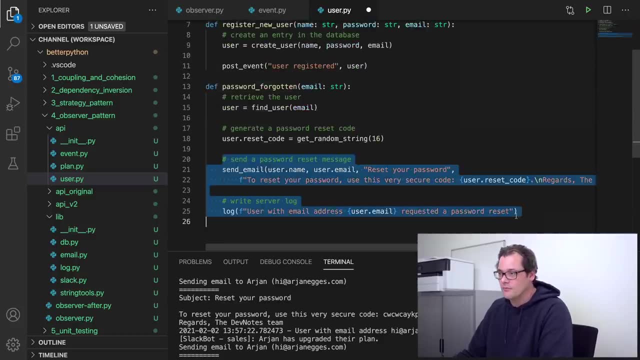 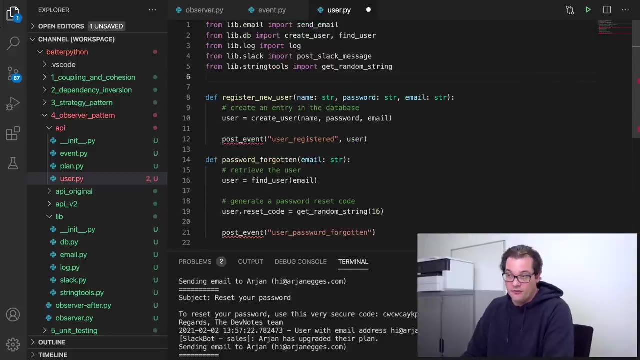 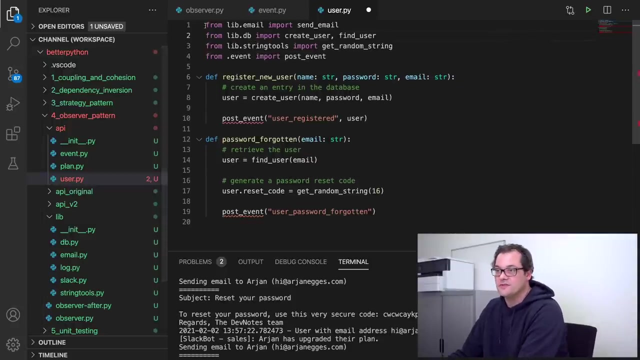 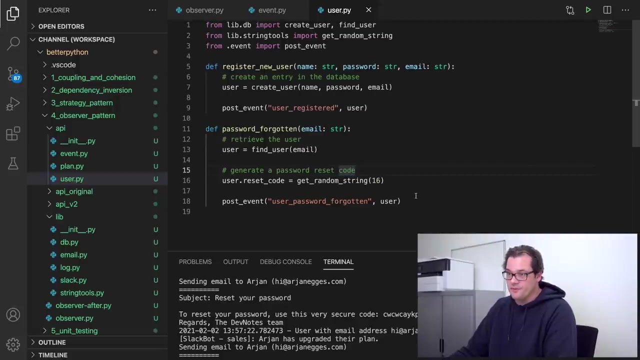 event call and as the data I'm going to pass along the user and same thing here. then, of course, I also need to update my imports, and now I can remove part of the imports that are no longer needed here, and I forgot to add the user there. so much shorter this way, and now what I can do is that. 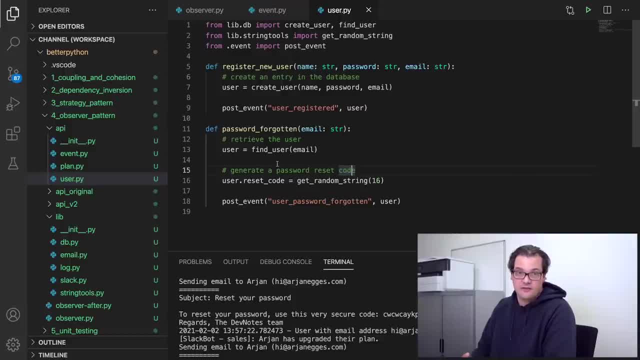 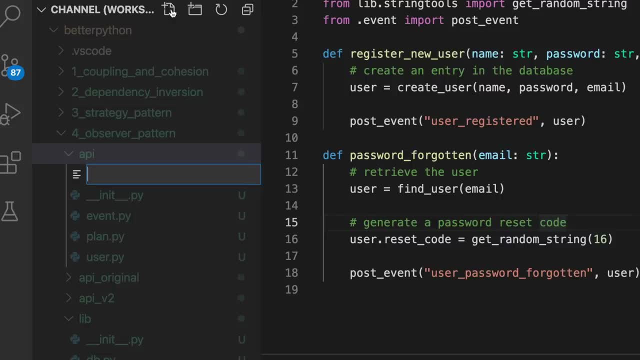 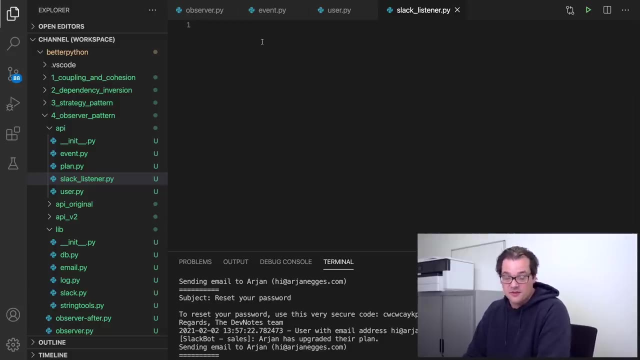 I can kind of group these different event handlers together in the way that makes sense. so, for example, I could add here a slack event handler, so create a file slack listener. then what I'm going to do is import this post message that I'm mainly going to use to do that, and of course I need the. 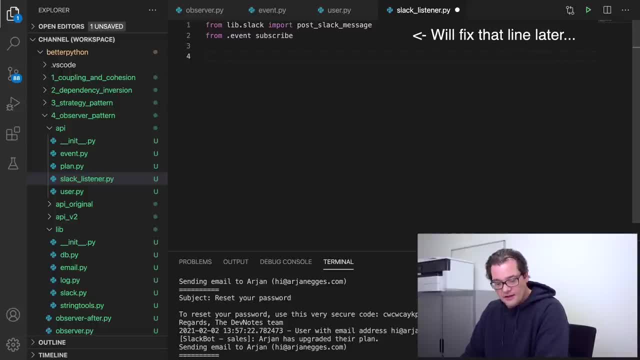 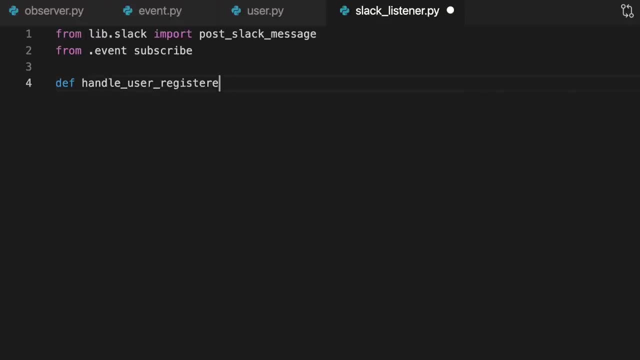 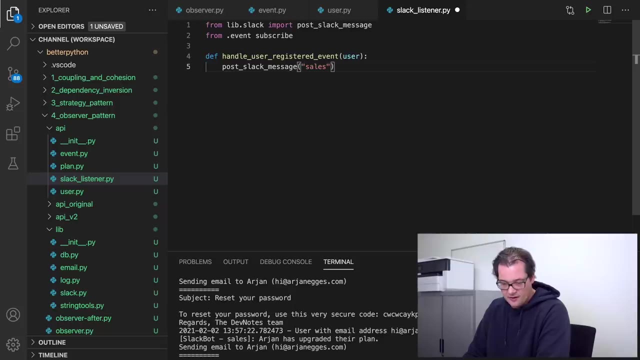 event library. and then, first thing is, let's add a function that handles a user registered events, and there we're going to put the slack message to sales and, of course, don't forget to spam this person. there you go, so we have our handle user registered event. no, got an import here and most 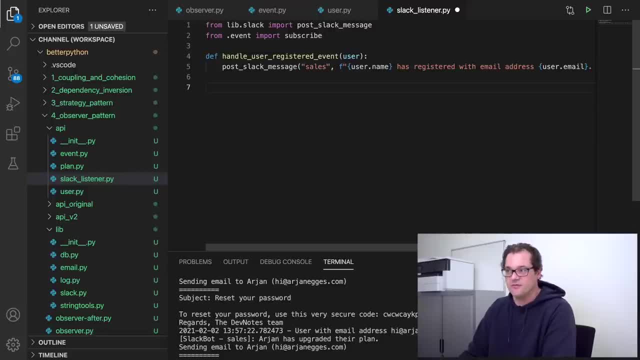 important here is that we need to be able to see our event library right here going to add a function that sets up the event handling system for Slack messages and that's gonna call the subscribe method. that subscribes us to particular type of event and then user registered event should be mapped to the 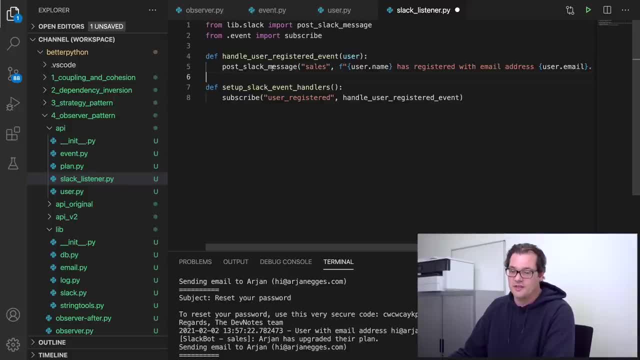 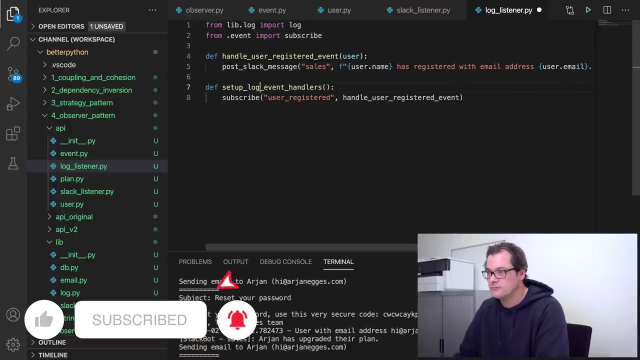 handle user register event function, and now I can add more functions here, like when the user upgrades the plan, etc. etc. now in a similar way I can do that for, for example, the system logs. so at the log listener file I'll just copy this over, because I need to do a lot of things the same and now I'm not posting. 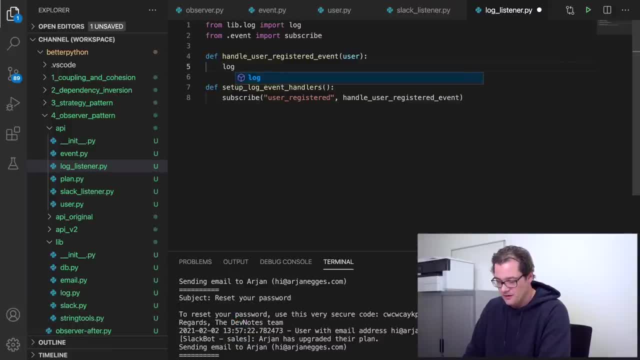 a slack message, but I'm sending a system log event and I can do the same. let's say, I want to add a, a password forgotten event like this, and they add a subscribe method call here. so I created these two collections of listeners and in the observer I then 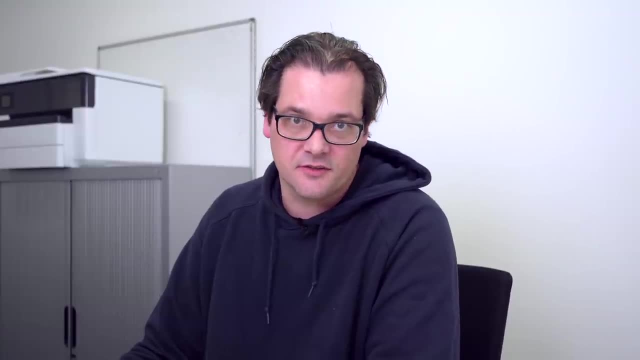 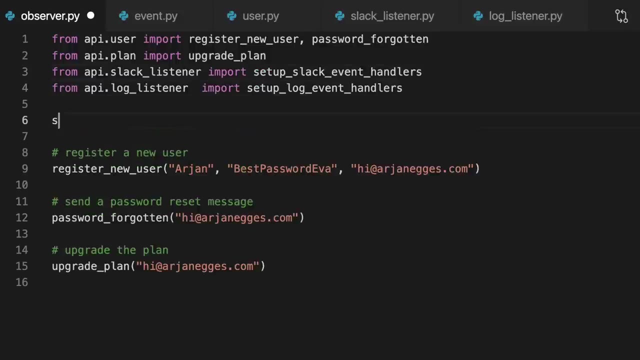 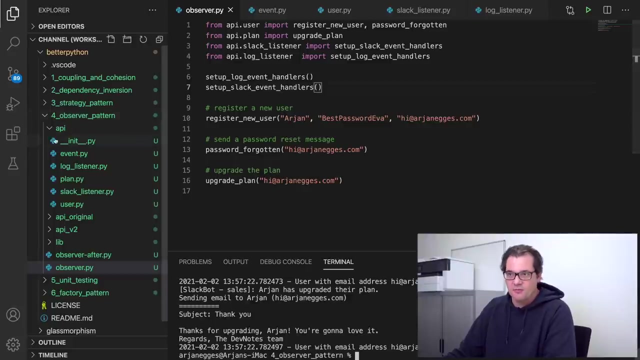 should import those and call this function so that the event system is set up correctly. so I'm not going to show how this works for all the functions and all the methods in this particular example, but I made a kind of complete version of this example where I rewrote this API. 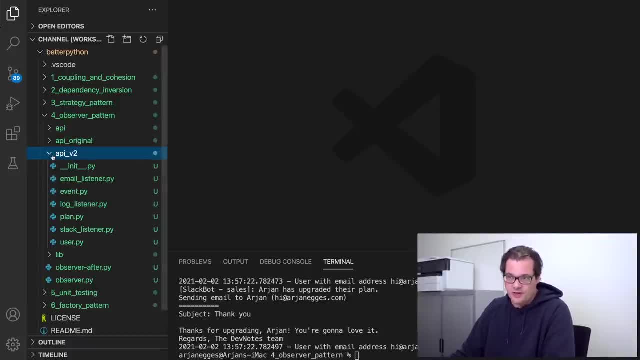 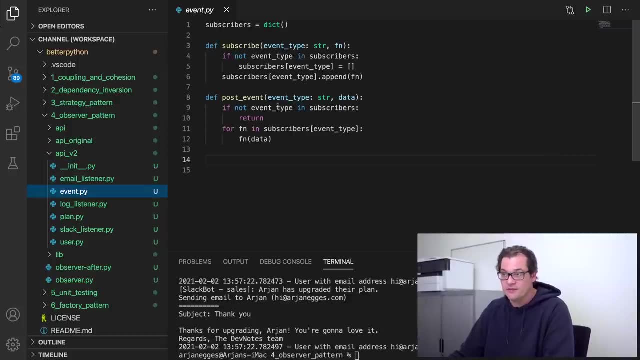 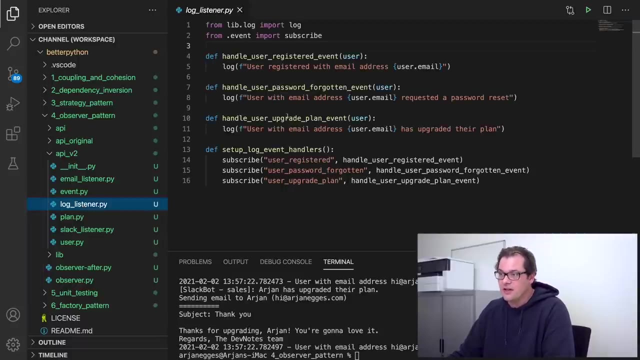 so that it now uses this event system. that's also in the same repository. so if you check it out on github, you can look at it and play with it yourself. so you see, we have here this event system that I just added, and we have a log listener with a couple of different event handlers and we have slack. 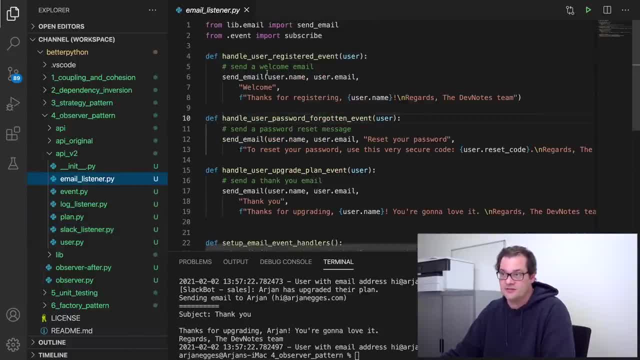 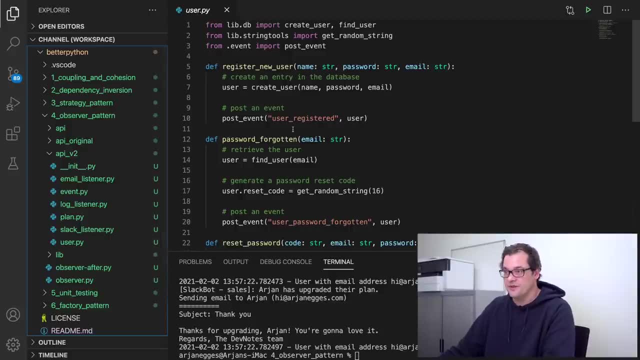 listener that looks the same and we have an email listener that actually sends the emails and the user and plan API access points now simply post an event instead of using directly sending emails, posting logs or posting slack messages, and something really interesting happened here. if you look at the way that it's now structured and 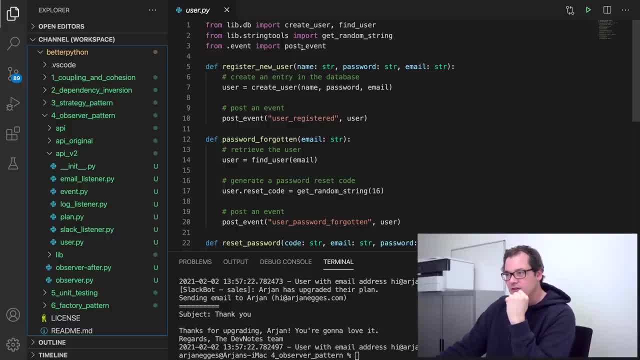 the way that the imports are organized. is that? here you see that the only dependency is on the event system. there's no longer any dependency on the type of specific type of message or specific type of things you want to do, depending on the event that occurs, and the same is for the plan. 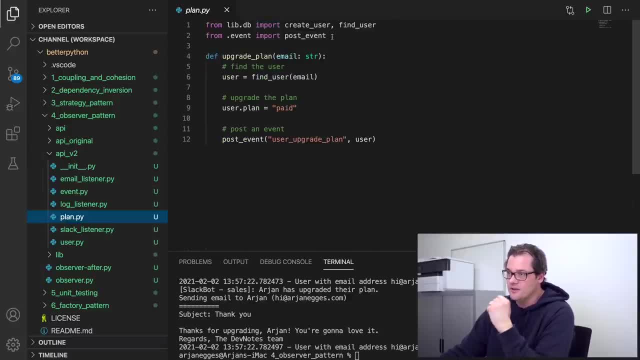 so there's, there's just the database stuff and the event stuff, that's it, and the methods are also becoming much shorter, so we just have to make sure that we have all the things that we need to do, and so we just have the database operation and then we post the event. if you look at the listeners, 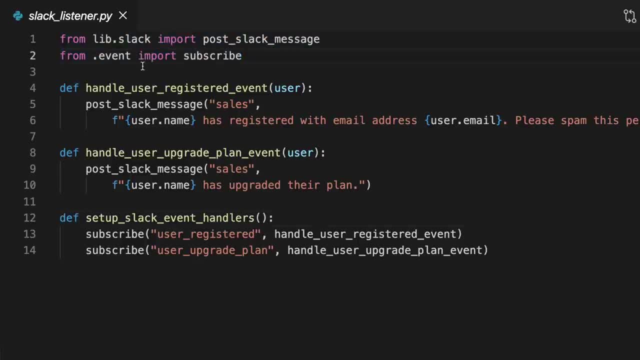 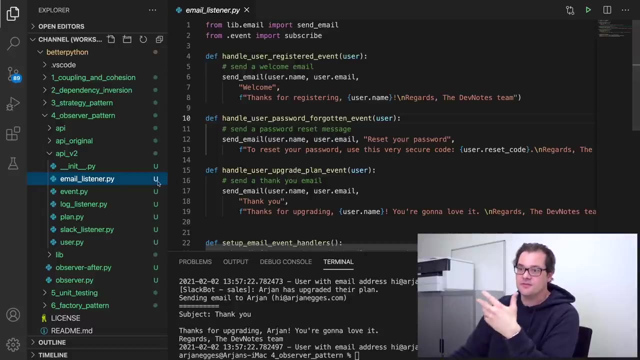 themselves. you also see that the number of imports is actually pretty low. it just imports event stuff that it needs and since this is a slack listener, it needs to post slack message import, and the same for the log and for the email. so using the event system in this way has allowed us to really 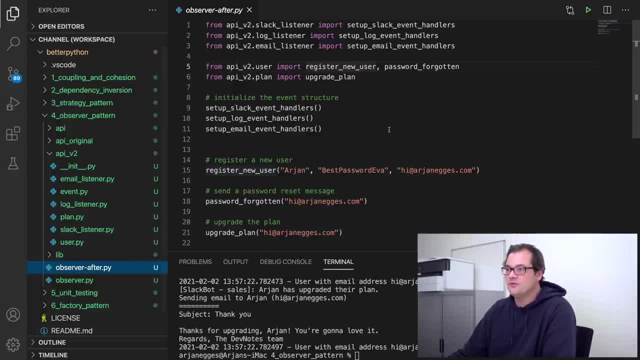 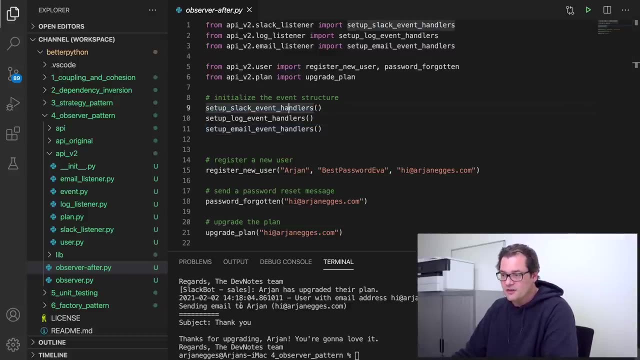 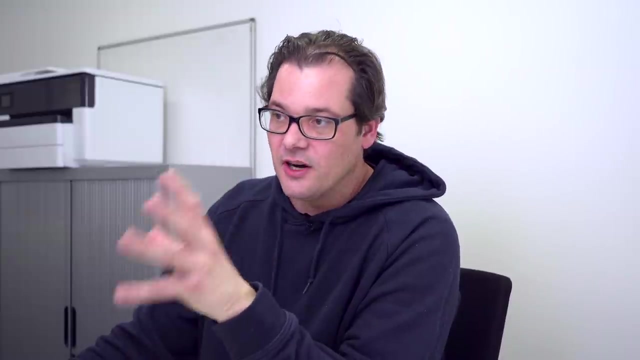 separate the code much better if you look at what we do in the actual test program. so we're simply initializing the event structure by calling up these event Handler setup functions and then when I run this, you see that it generates a bunch of emails, slack messages, log messages, Etc. when I call these functions here and now. it's really nice that not only are the 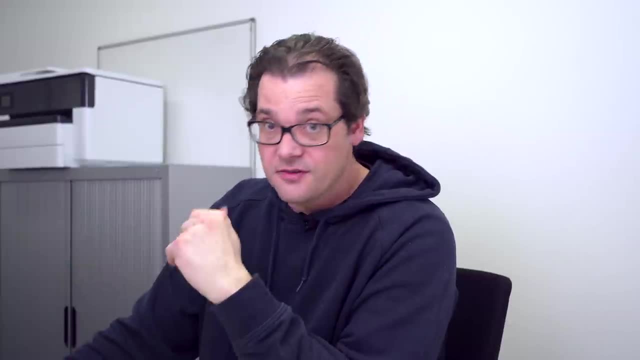 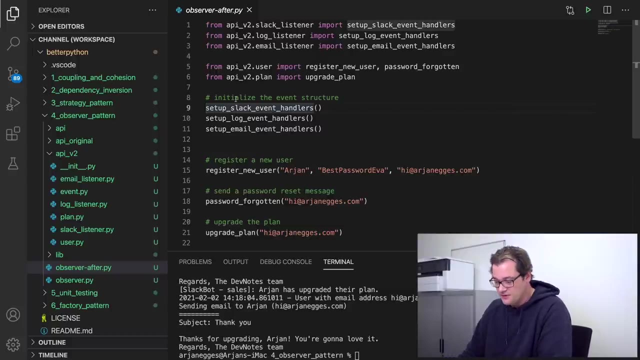 imports much better structure that has less coupling. because of that, some things are now much easier to change. so, for example, if I want to temporarily disable slack messaging, I could simply put this into comments and if I run the code again, there are no more slack messages. I 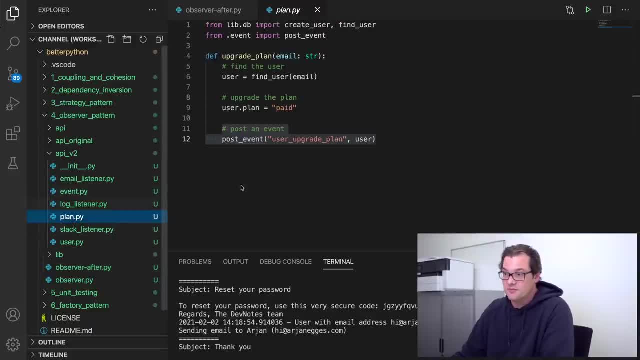 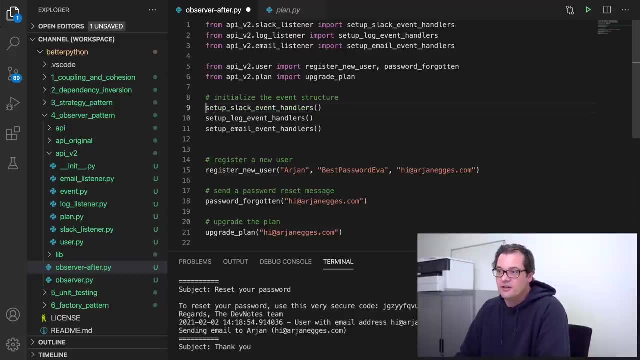 didn't have to change anything in my actual API functions, because these simply post an event and don't know anything about what happens after that. now, similarly, if let's say I wanted to change from slack to a different message provider, like Microsoft Teams or whatever you use in your 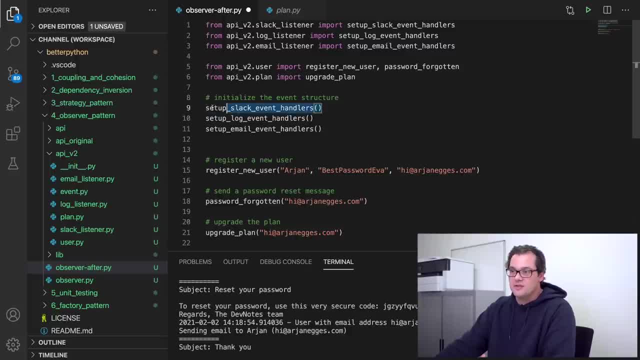 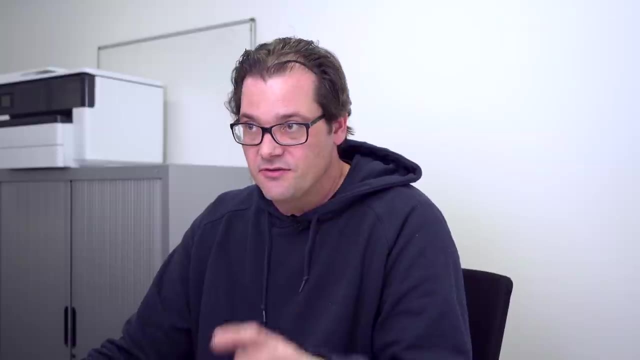 company then also. that would be a pretty easy change. I would simply disable this and then add a new listener for my new messaging service and enable event handling and I'm basically done. I don't need to change anything else in the code. in the previous version I would have to sift through. 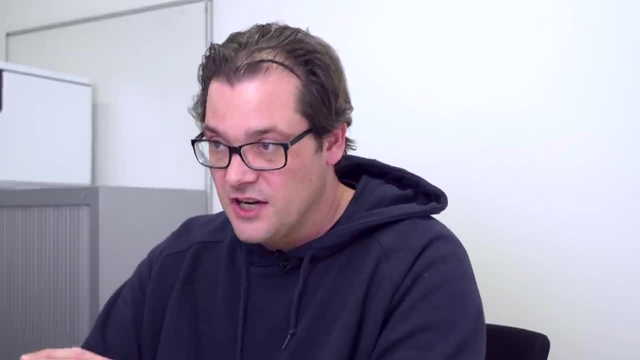 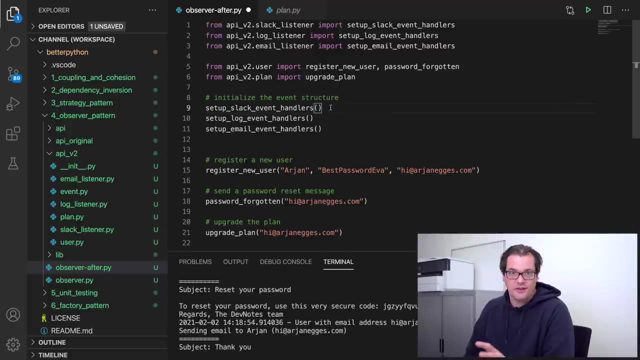 each of the functions in my back-end service and change the slack specific part to a team's specific part. so there you see a very clear example of how reducing coupling helps you write code that's much easier to change later on. and this event mechanism- I said it before- it's 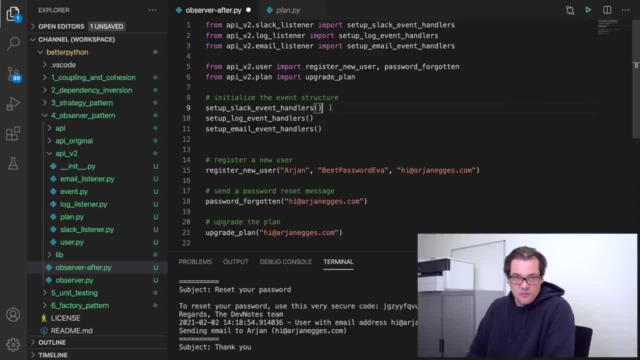 really really useful for these kind of things, and a lot of people only use events for UI stuff like handling a button click or stuff like that. but just keep in mind that if you encounter this kind of structure or this kind of thing in your code, that events can really help to clean it up. you know, on this, 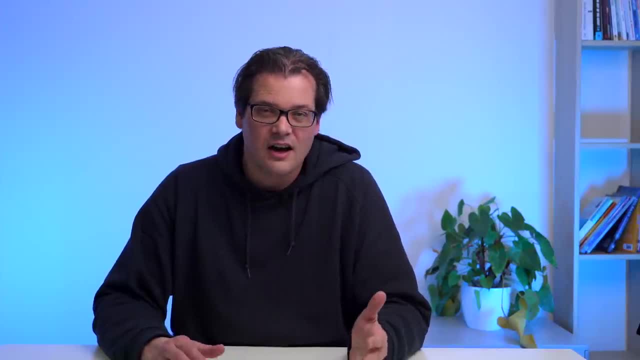 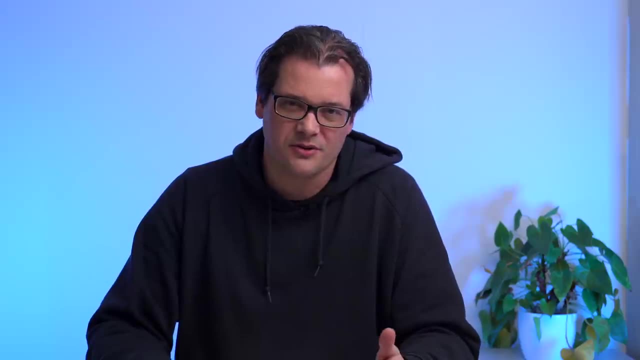 channel. I like to talk a lot about writing code and designing software. I don't like to just provide recipes like how to do X, but I'd like to think a bit more about why we're doing things the way that we do them. I've been teaching computer science. 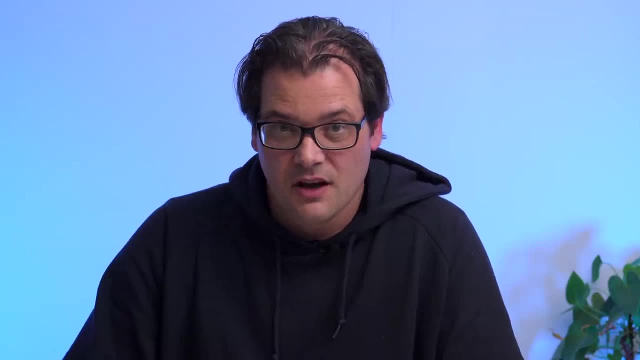 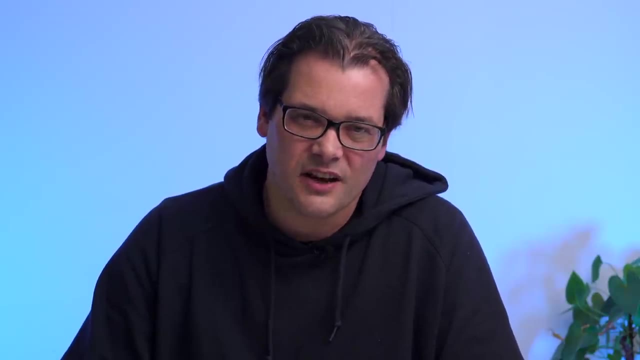 for over 20 years and I've started several software businesses, and simply following recipes never really led to good results for me. I really needed the understanding that's behind it. on the other hand, there are lots of tutorials out there about design patterns and design principles, but 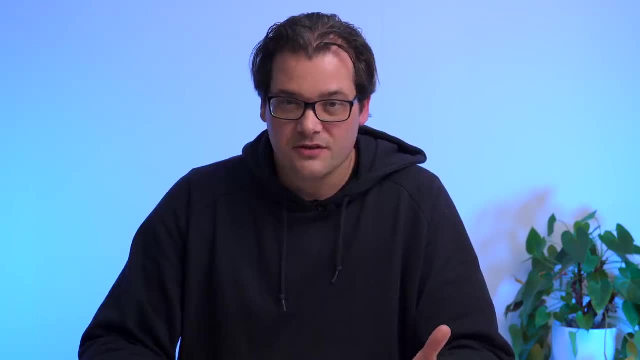 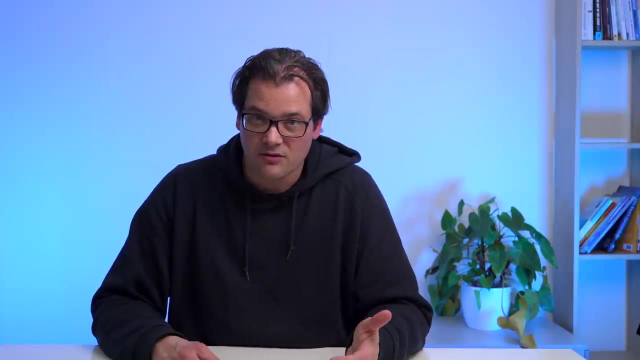 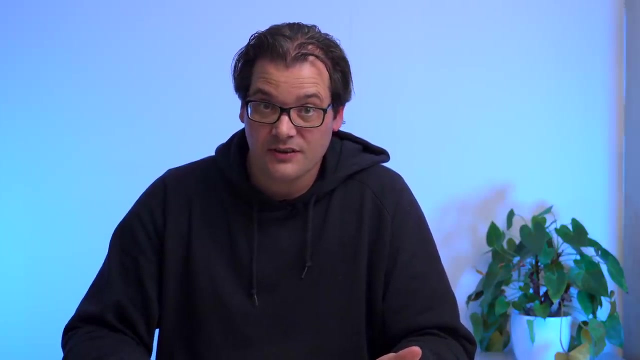 often the examples are not very practical. what I discussed today was a solution to a problem that I literally had a few weeks ago. I hope this video helps you think differently about how you write code. let me know in the comments below what your thoughts are about this. you can find a link to GitHub repository containing the code that I worked. 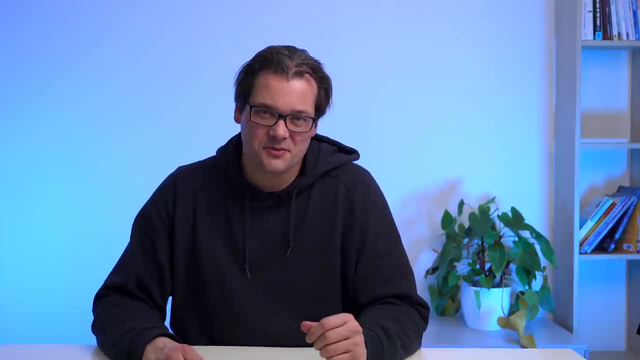 on in this video in the description below. if you're enjoying this series, consider subscribing. thanks for watching. take care and see you soon. 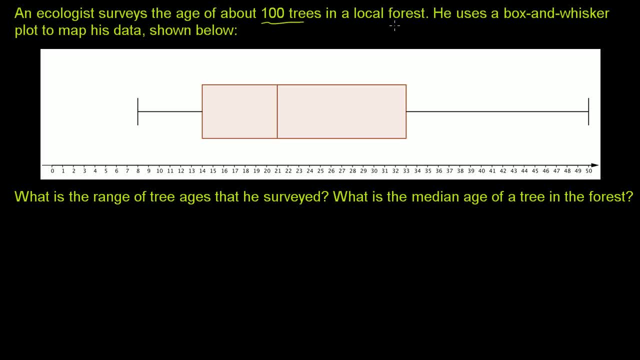 An ecologist surveys the age of about 100 trees in a local forest. He uses a box and whisker plot to map his data, shown below. What is the range of tree ages that he surveyed? What is the median age of a tree in the forest? 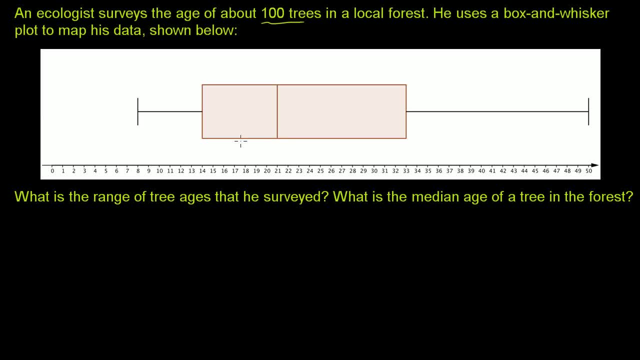 So, first of all, let's make sure we understand what this box and whiskers plot is even about. This is really a way of seeing the spread of all of the different data points which are the age of the trees, and to also give other information. 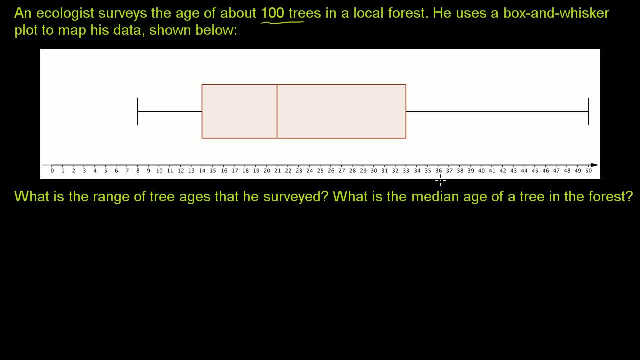 like what is the median and where do most of the ages of the trees sit? So this whisker part- so you can see this black part- is a whisker. this is the box, and then this is another whisker, right over here. 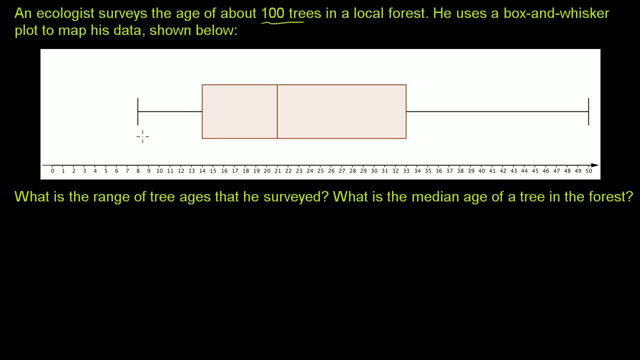 The whiskers tell us essentially the spread of all of the data. So it says the lowest data point in this sample is an eight-year-old tree- I'm assuming that this axis down here is in years- And it says that the oldest tree right over here is 50 years. 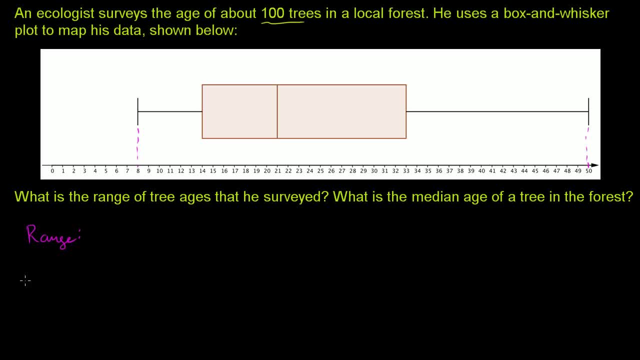 So if we want the range- and when we think of range In a statistics point of view, we're thinking of the highest data point minus the lowest data point, So it's going to be 50 minus 8. So we have a range of 42.. 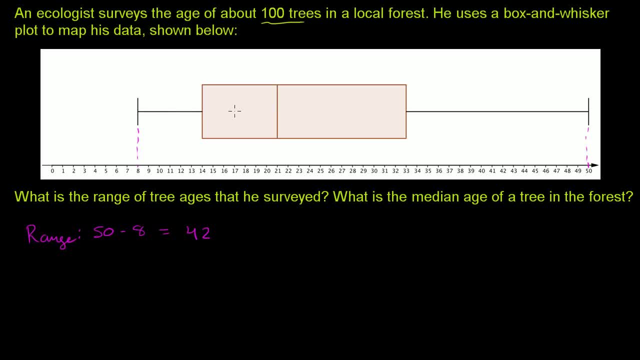 So that's what the whiskers tell us. It tells us that everything falls between eight and 50 years, including eight years and 50 years. Now what the box does? the box starts at. well, let me explain it to you this way.